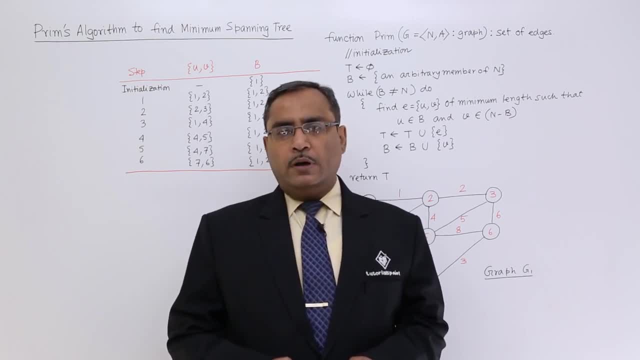 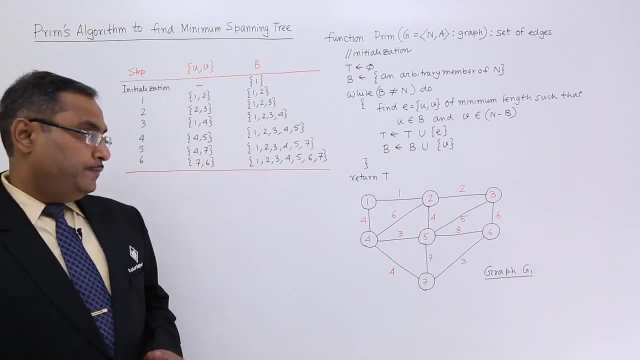 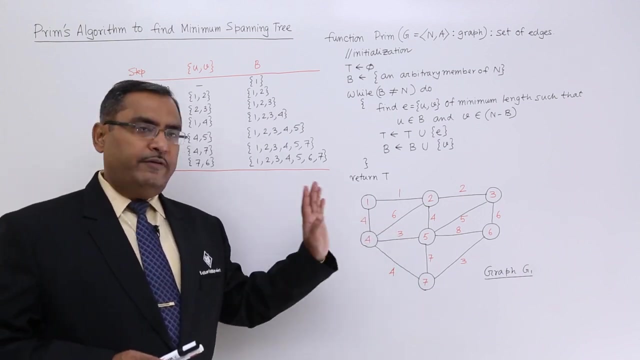 Now let us execute Prim's algorithm on a given graph. Now see, this is a graph given. So graph G1, it is having 7 nodes and it is undirected weighted graph. So these are the weightages given. So this is my Prim's algorithm. I shall execute my Prim's algorithm on this. 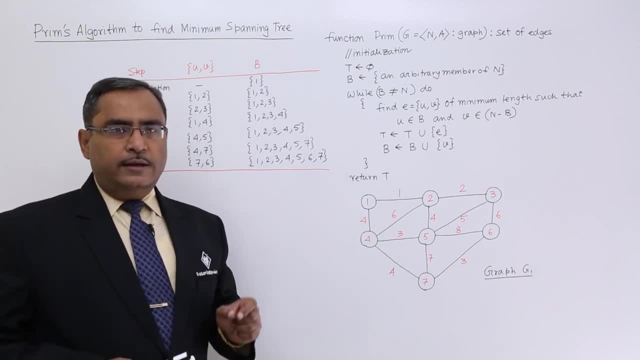 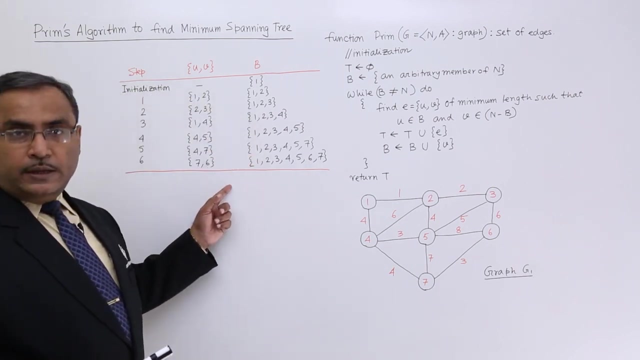 particular given graph with the seed element as 1.. So seed element means the first element from where the minimum spanning tree will grow. So that seed element has been supplied, Let us consider, let it be 1.. So now, this is my tracing, So we shall. 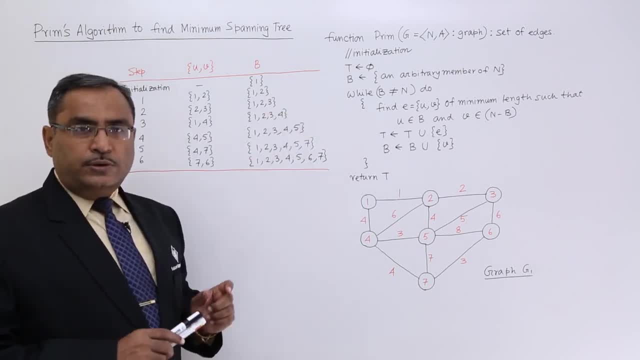 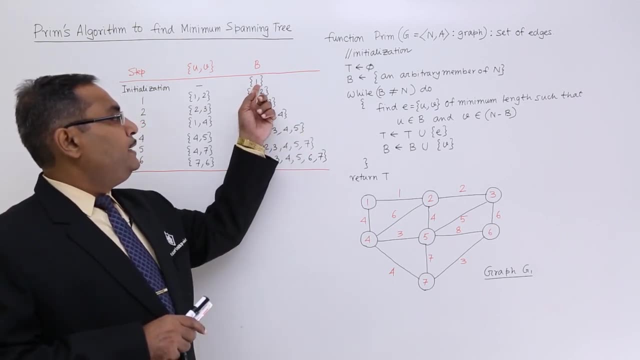 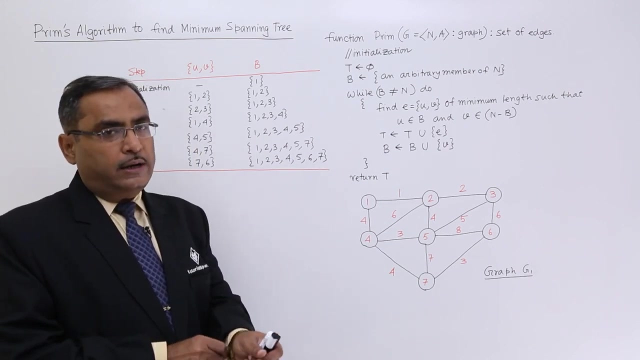 go for this. Now t is equal to phi. So at first the t is equal to phi is there, and then we are having this B, an arbitrary member of N. So B is having 1 at first, as we have planned that B will be having the seed element at first, So that is 1 in this case. So 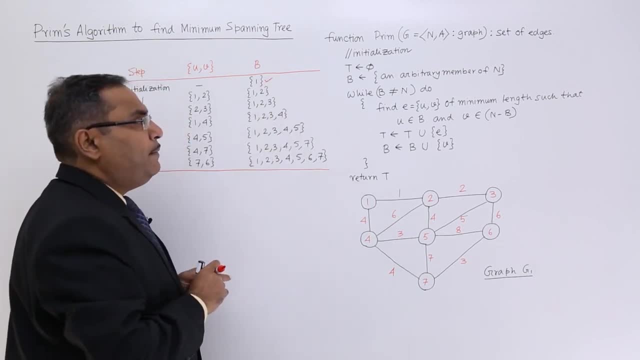 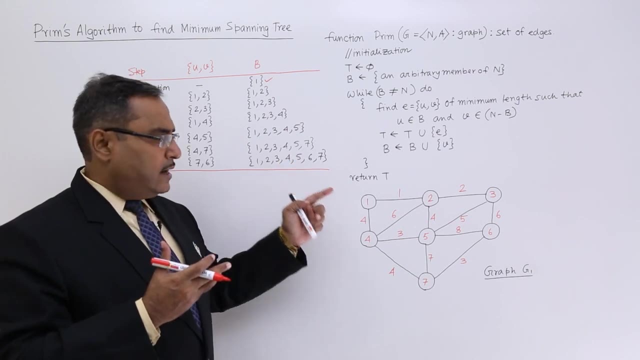 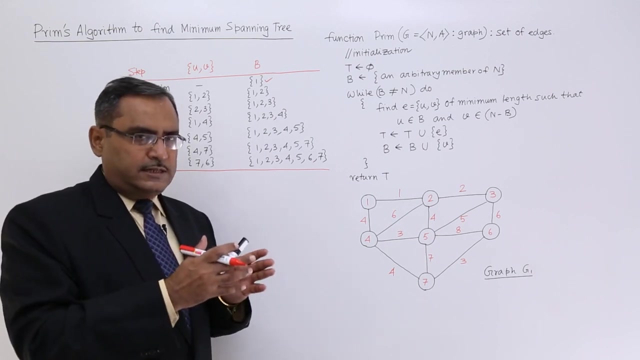 we have discussed this one, While B is not equal to N. So until B is going on including all the vertices. How many vertices are there? 7 vertices. So until B is accumulating all the 7 vertices inside. So this algorithm will be continued. Find E, U, V of minimum. 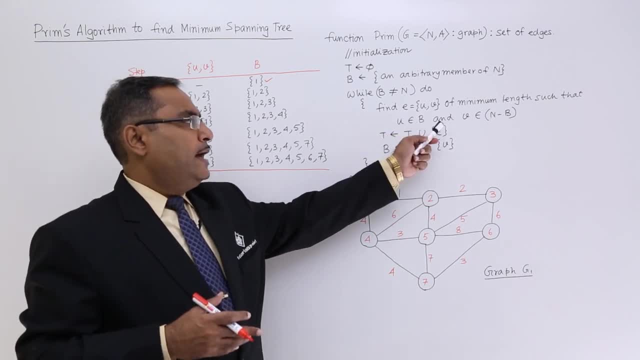 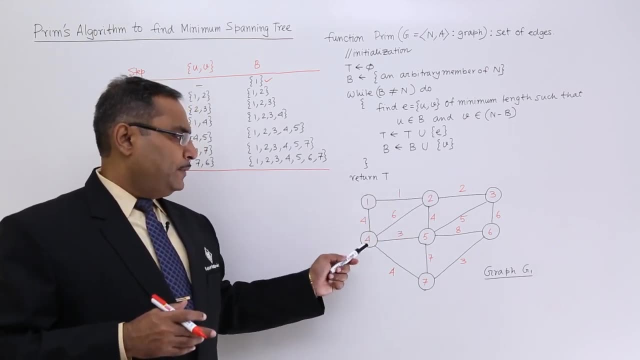 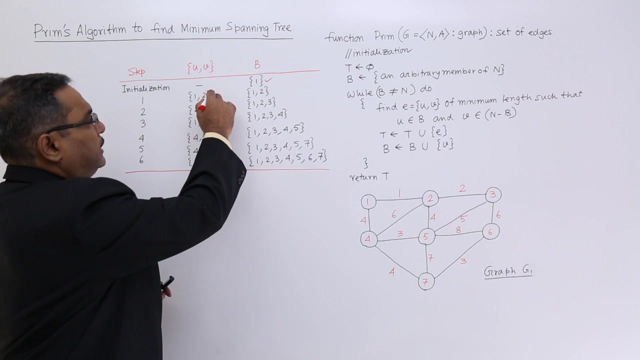 length, such that U will be belonging to B and V will be belonging to N. So this is N minus B. So now you see from 1, what is the minimum weightage age you are having. So I think that is 1.. That is 1, 2.. So I should consider this particular age and this: 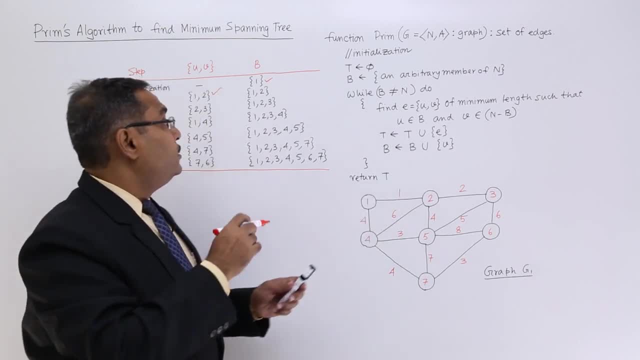 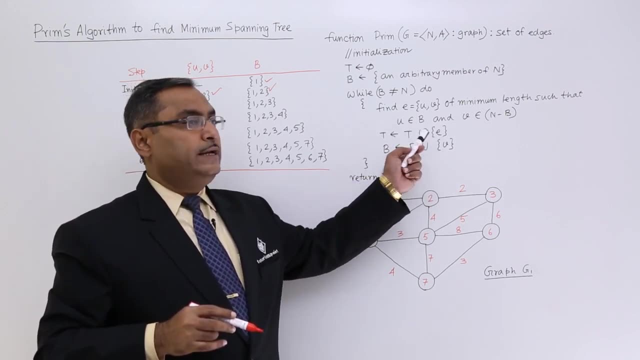 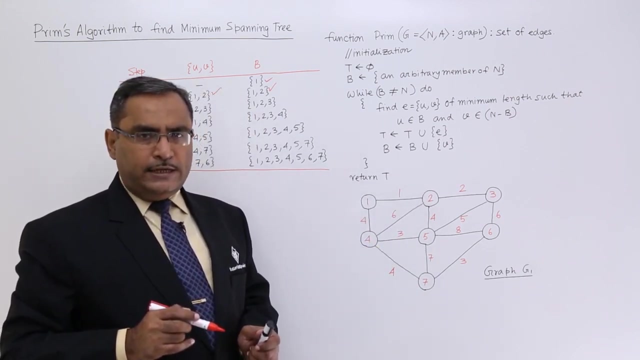 particular new node will be included in B. So 2 has got included in B, union in B with B, and now t is equal to t union E. So this is the age we have considered, Next from 1 and 2, what is the minimum age we are having? So, from 1 and 2, we are having 2, 3 with the. 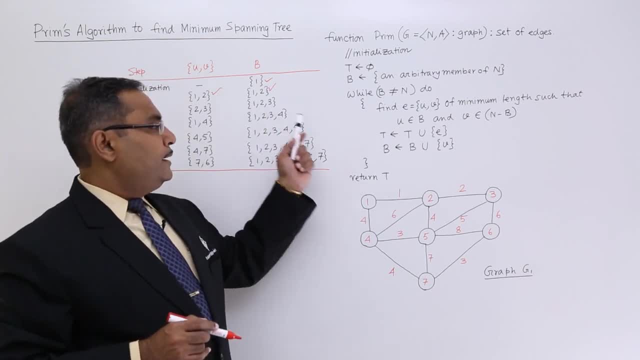 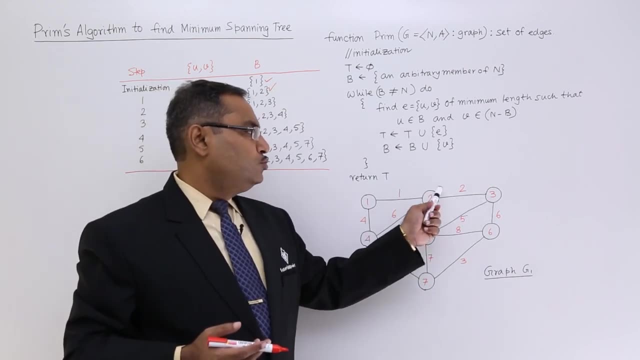 weightage of 2.. You see, 2 is included in B, but 3 is not included in B. Obviously, 3 is in N. So that is why we should consider this one, So 2, 3.. So next age will be 2,, 3 and. 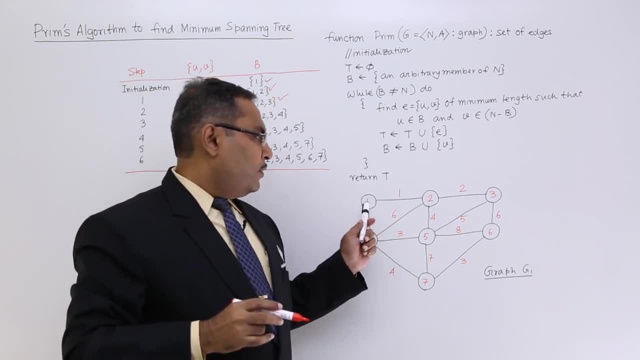 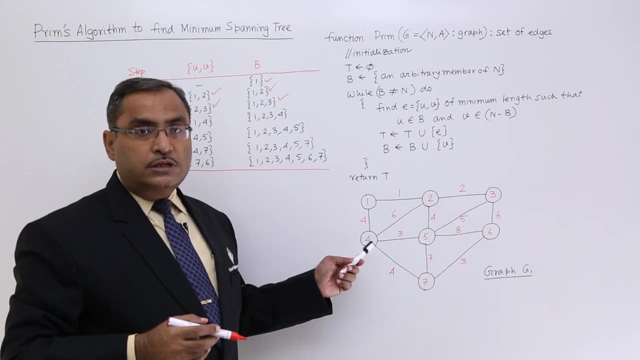 this 3 will be union with this B. So from 1,, 2, 3, what is the outward age? What is the age which is connecting another uncommon node, Unconsidered vertex? So here we are having 1, 4.. Also, we can have another tie has occurred. 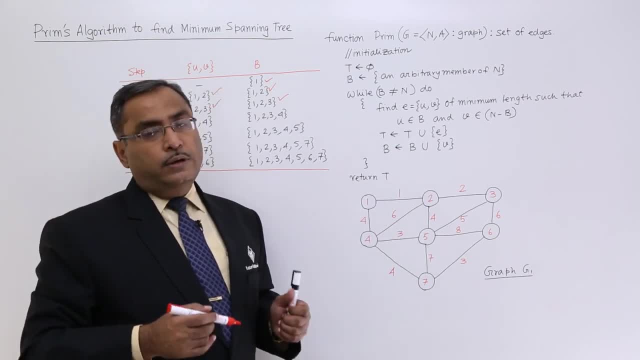 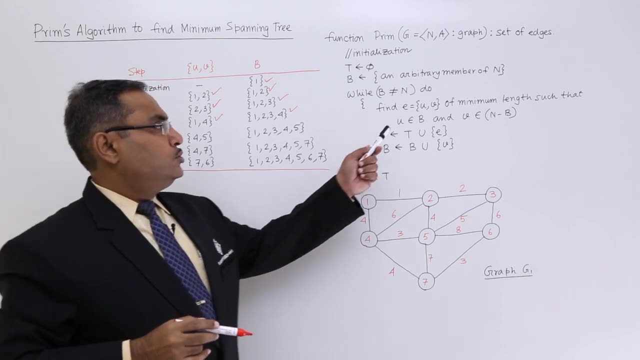 So that is my 1, 2, 5.. So that is why we can resolve the tie arbitrarily, So I shall go for 1, 4.. So 1, 4 has been taken and 4 has been unioned. So you are taking this. 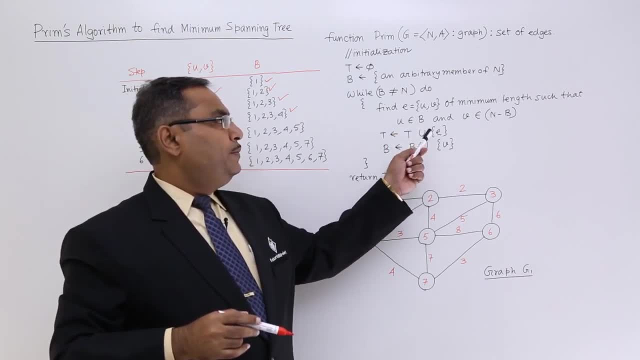 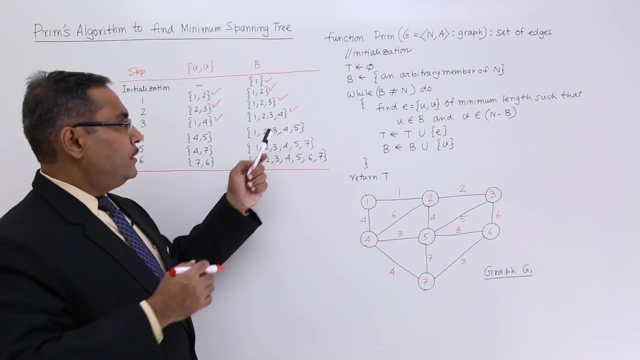 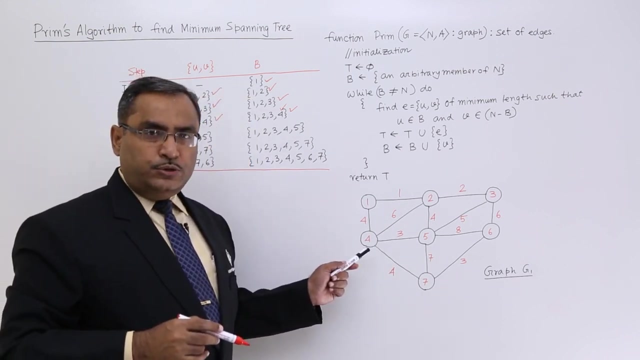 1, 4.. So this particular age will be union with the solution t and this 4 will be union with B. So that is why 4 has come here. So 4 is the new node. Now, from 1,, 2,, 3, 4, what is the age we should take? I think that is 4, 5.. I think that is. 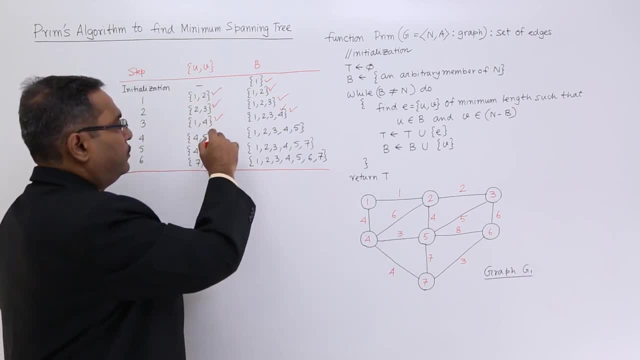 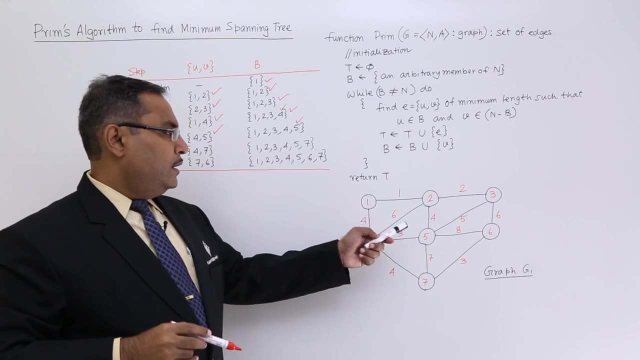 4, 5 with the weightage of 3.. So we are going for this. 4, 5 and 5 will be unioned here. So now we are having this: 1, 2, 3, 4, 5.. From 1,, 2, 3,, 4, 5: what is the age? What is? 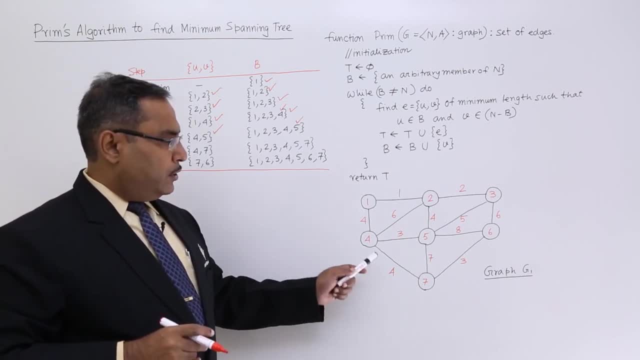 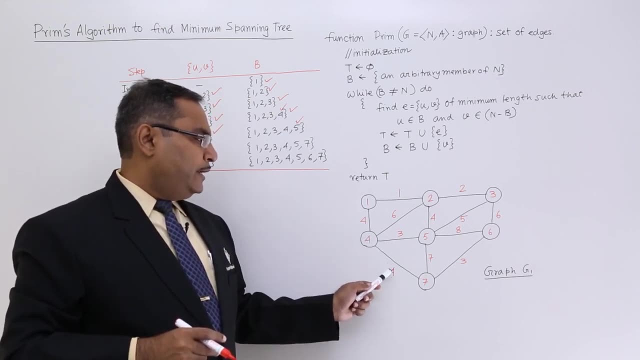 the age we are having and that is the 4, 7.. That is the 4 because 1,, 2,, 3,, 4, 5 we are having this 4 because 4 is connecting This particular weight. age is in between the nodes 4 and 7. 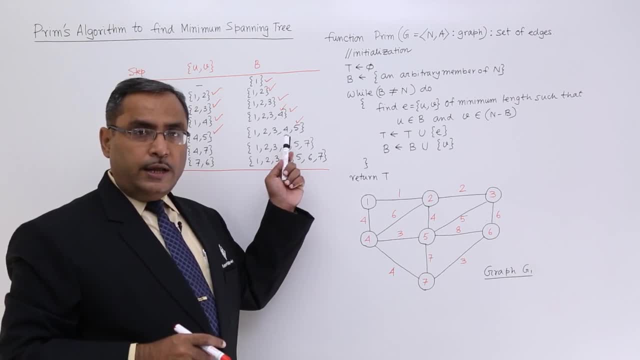 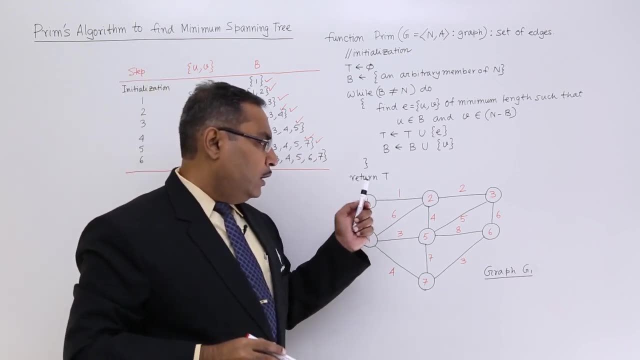 where 7 is not already there, but 4 is already there in our B, So we shall take this: 4 and 7, and 7 has got included accordingly. So now we are having 1, 2, 3, 4, 5, 7, 1, 2,. 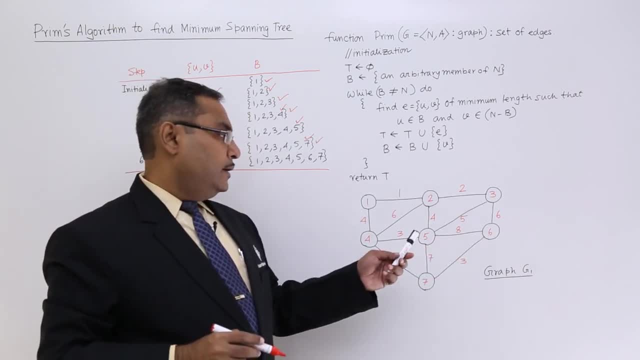 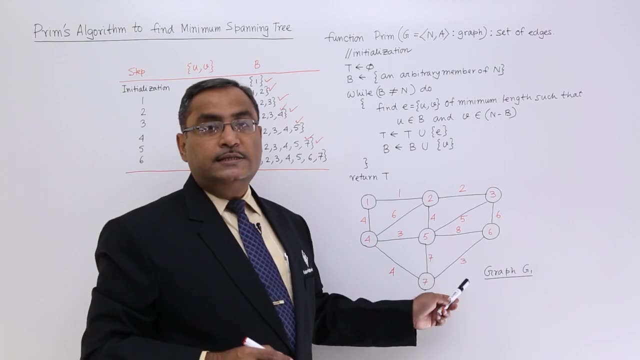 3,, 4,, 5, 7 and 6 is the only node we are having, So which is not included in B, here this weight age is 8, here this weight age is 6.. and here this weight age is 3.. So I should consider this age 6, 7.. So I should consider. 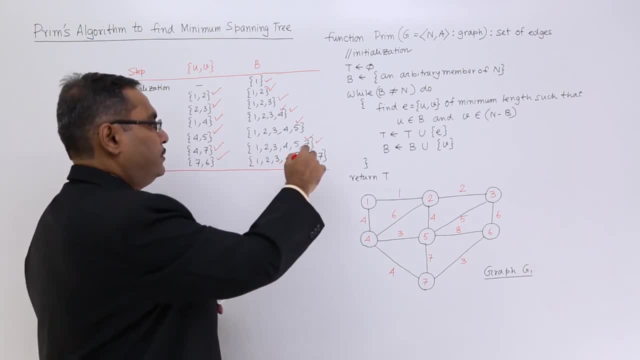 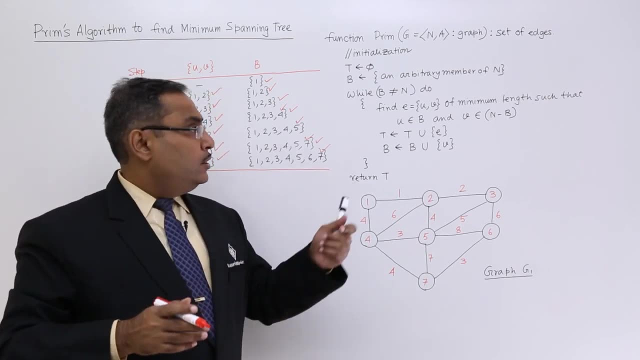 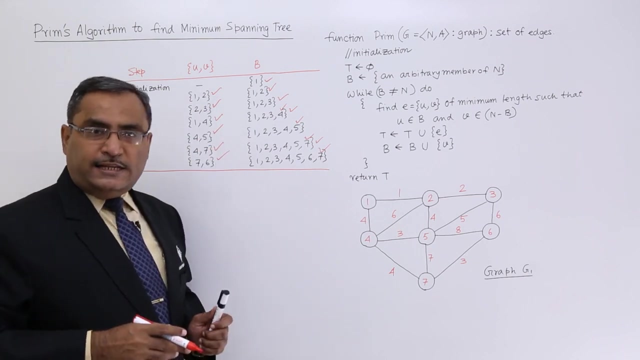 this age 7, 6 or 6, 7, because they are undirected, So I am just taking this one here. So now you see, b has grown, which is equal to n. So this particular while will terminate and this return t. So these are the respective ages in the t and they will be returned and that